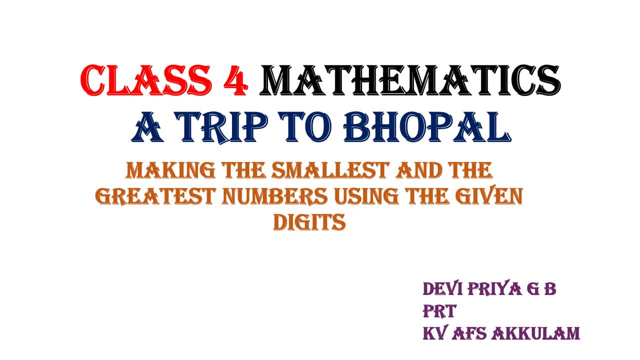 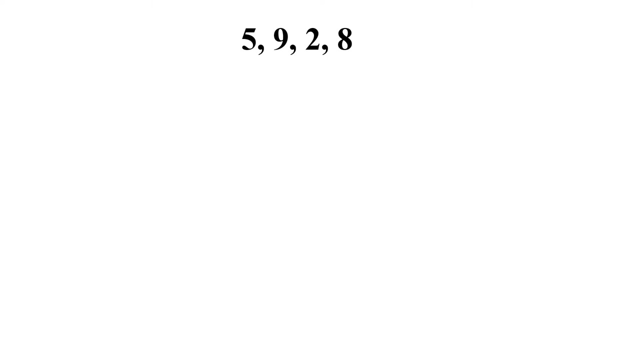 Welcome to class 4 mathematics Chapter. a trip to Bhopal. Topic: making the smallest and the greatest numbers using the given digits. Children have a look at these numbers. Which is the biggest among these numbers? Yes, it is 9.. Can you tell which is the smallest number? 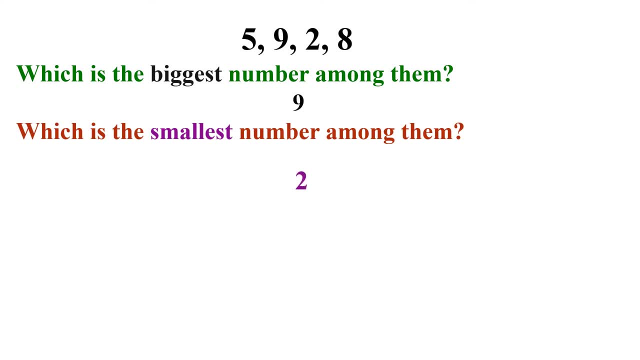 Yes, you are right, It is 2.. Now read this question. Write the smallest and greatest four-digit number using all these digits, without repeating, To find the smallest four-digit number, you have to write the numbers in ascending order Here. when you write the ascending order, it is like this: 2, 5, 8 and 9.. So write these numbers. 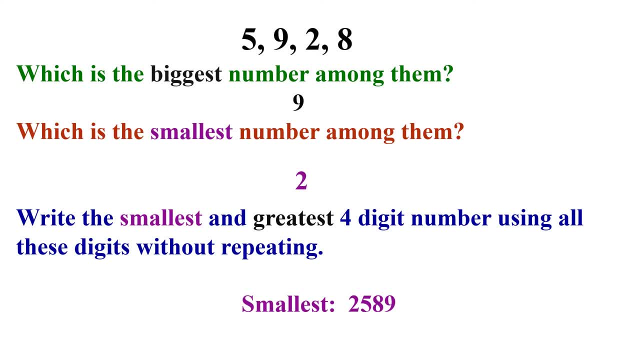 without comma, and the number will be 2589.. This is the smallest four-digit number. And what about the greatest four-digit number? You have to write the descending order of these numbers, That is, 9,, 8,, 5 and 9.. So you have to write the descending order of these numbers. 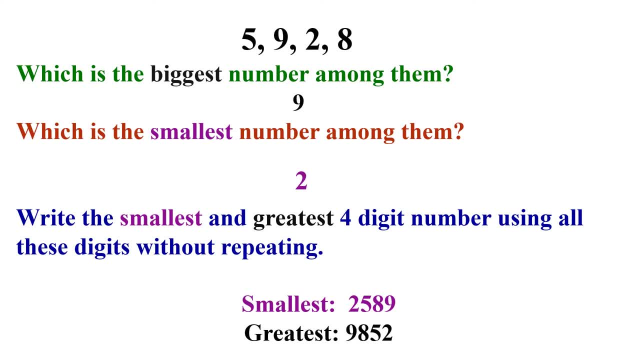 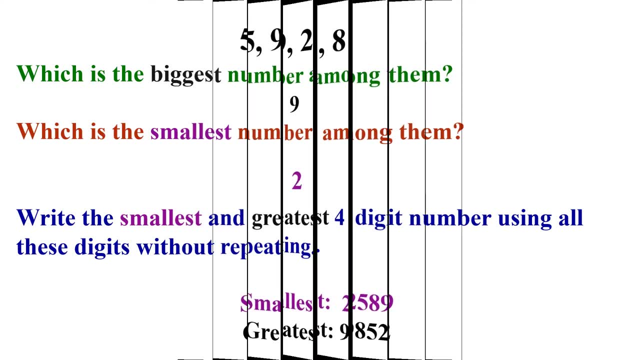 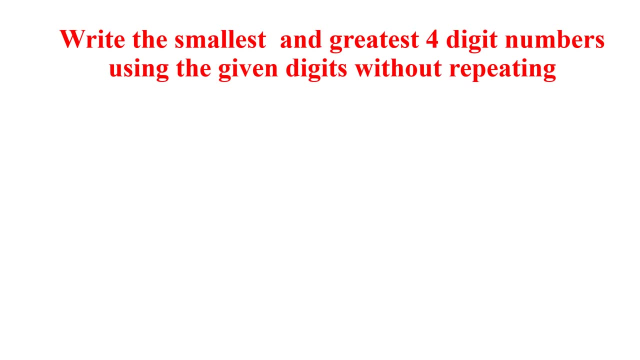 9,, 8,, 5 and 2.. 9, 852 is the greatest four-digit number. here Write the smallest and greatest four-digit numbers using the given digits, without repeating First question: 9,, 5,, 2 and 4.. In order to find the smallest four-digit number, 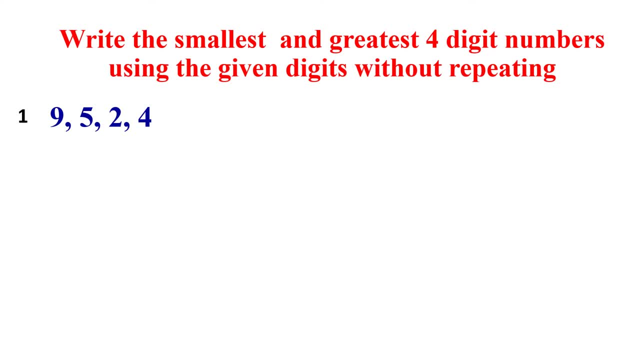 we have to write these numbers in ascending order, That is, from smallest to the largest. Ascending order will be 2, 4,, 5 and 9.. So the smallest four-digit number is 2459.. For finding the greatest four-digit number, we have to write these numbers in descending order. 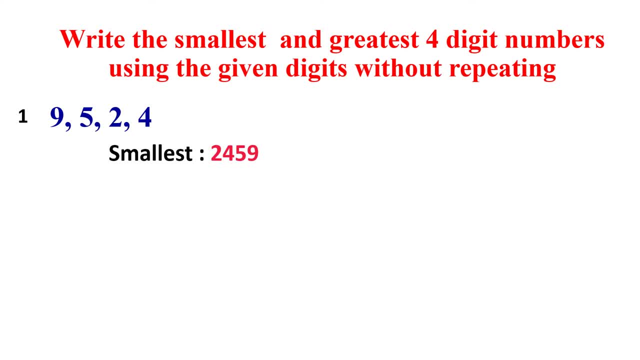 That is from bigger to smaller. The greatest four-digit number here is 9542.. Second question: 7,, 1,, 9 and 8. Here you have to repeat the same method. You will get the smallest four-digit number as 1789.. 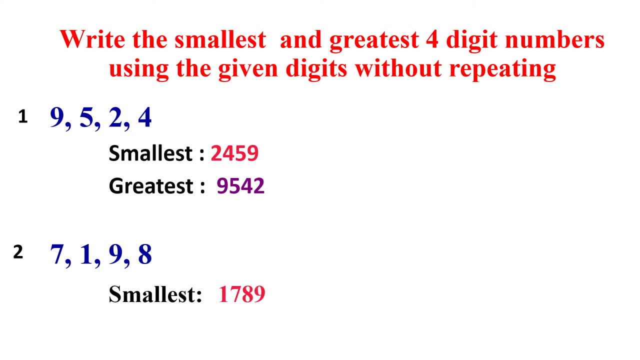 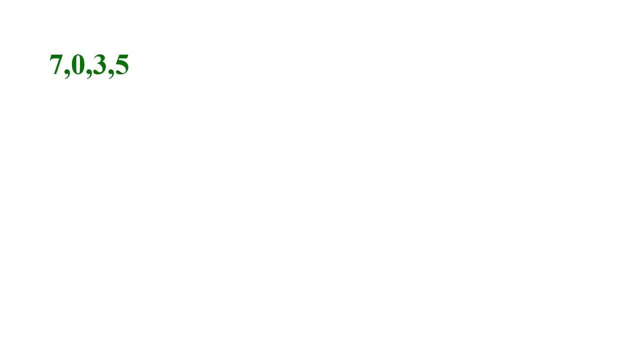 That is 1789, and the greatest four-digit number as 9871.. For finding the greatest four-digit number, you will get the smallest four-digit number as 9871.. Have a look at this question. For finding the smallest four-digit number, we know that we have to write in ascending order. 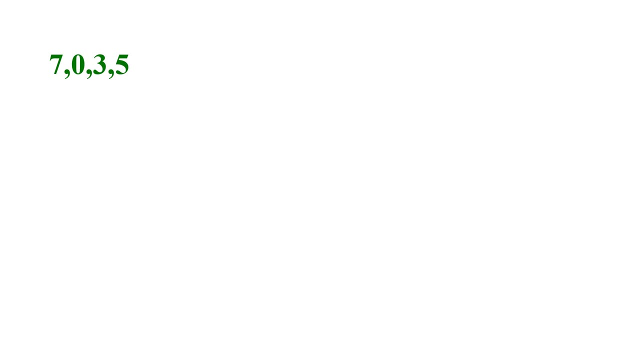 But look here You can see 0. here You should not consider 0 as the smallest number here, because no four-digit number can start with 0. So we have to write the smallest number other than 0.. 0 first. Here it is 3.. So we will start with 3.. 0 will be in the second position. 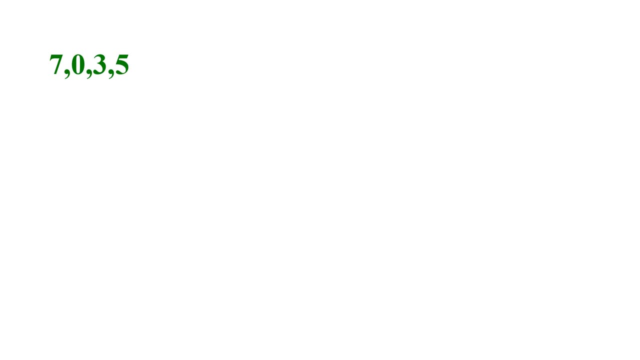 Then comes 5 and finally 7.. So the smallest four-digit number here is 3057.. Greatest number is, as you did earlier, That is in descending order. Here it is 7530.. Next question: 2650.. Here also there is a 0.. Can you tell me the smallest four-digit number here? 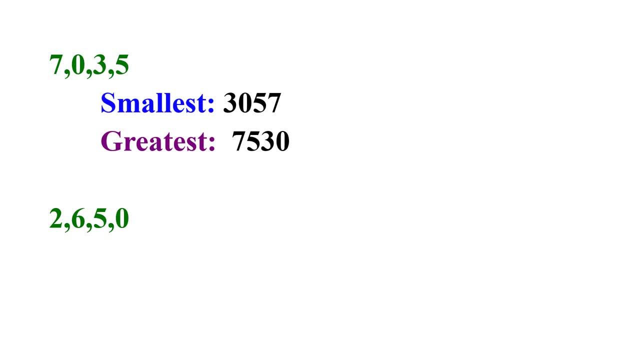 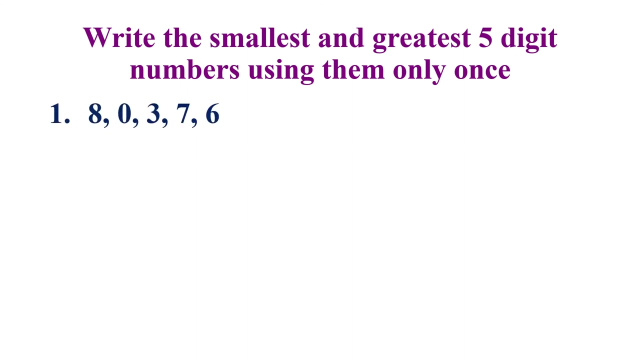 Yes, 0, to be written in second place only. So the smallest four-digit number here is 2056.. And greatest four-digit number is 6520.. Write the smallest and greatest five-digit numbers using them only once. First question: 8,, 0,, 3,, 7, and 6.. Instead of four digits, five digits are given here.